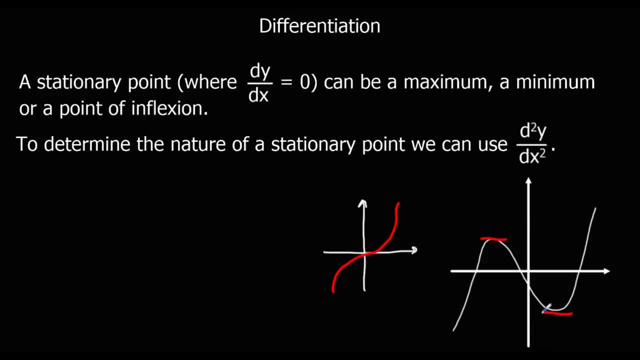 So a maximum is a top turning point, A minimum is a bottom turning point, And a point of inflection is where the gradient goes to zero, but then it carries on going in the same direction And we can determine the nature of a stationary point by looking at this: d2y, dx2, which means 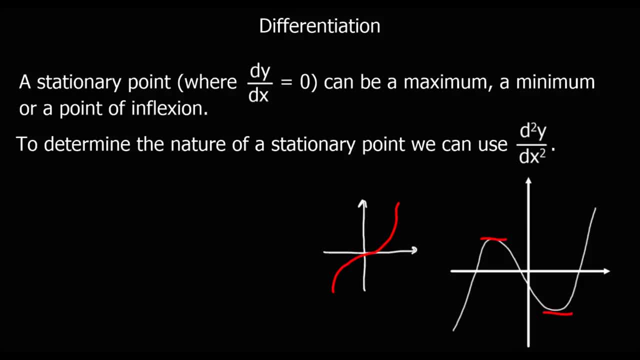 the gradient of the gradient. So we can look at the gradient of the gradient to find out whether it's a minimum, a maximum or if we don't know. So if I look at a maximum point here, the maximum point here, you can see that. 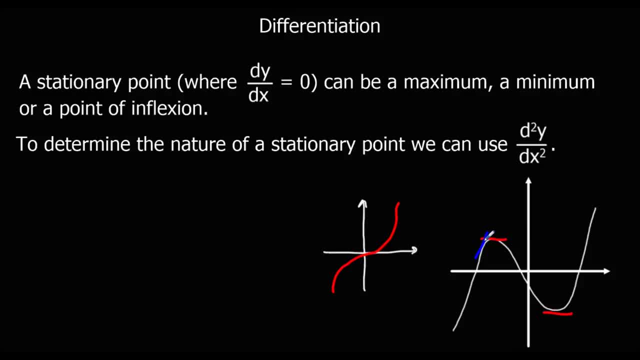 the gradient was positive and then it was zero and then it was negative. So the gradient is going down at a maximum. So the gradient of the gradient is negative. So if the gradient of the gradient is negative, that means I've got a maximum. 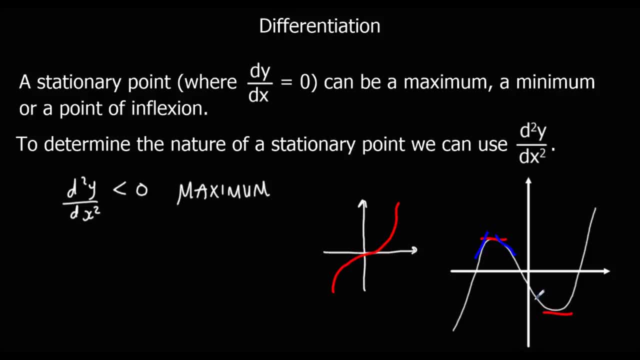 And if I look at a minimum, you can see that we've got a negative gradient and then it gets bigger. It ends up being a positive gradient, So that's increasing. So if the gradient of the gradient is going up bigger than zero, we've got a minimum. 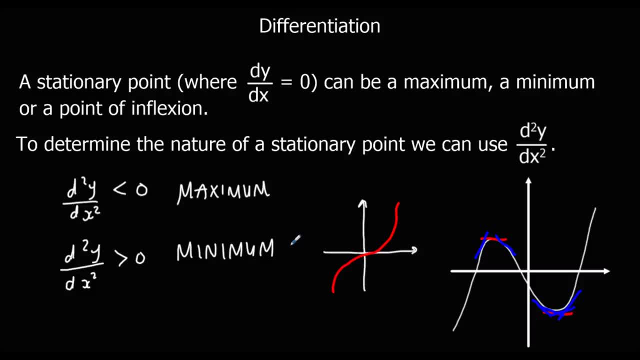 And if the gradient of the gradient is zero, that means we don't actually know. So it could be a maximum, a minimum or a point of inflection. So if I look at a maximum, I can see that the gradient of the gradient is positive. So if the gradient of the gradient is negative, we've got a maximum. 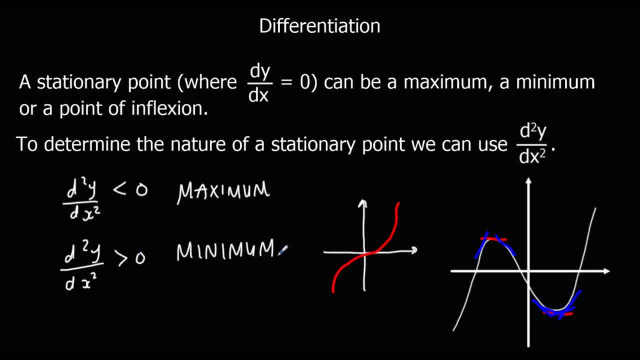 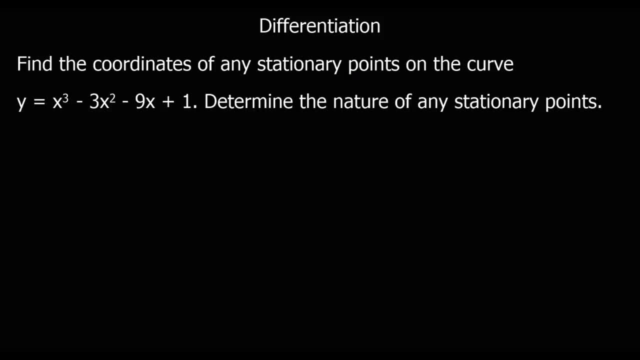 If the gradient of the gradient is positive, we've got a minimum, So we can use this to work out the nature of a stationary point. Okay, here we've got a question: Find the coordinates of any stationary points on this curve and determine their nature. 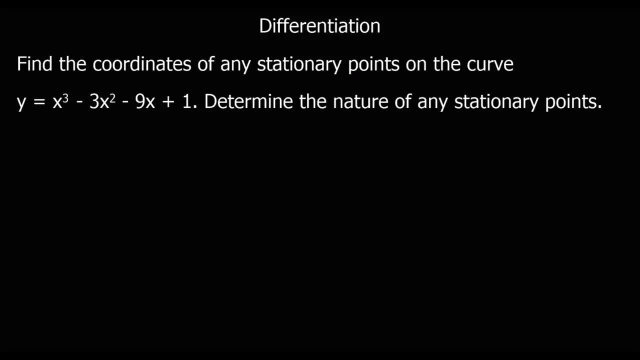 So to find the coordinates of the stationary points. stationary points are where dy dx is zero, where there's no gradient. So we're going to find dy dx, make it equal to zero and find out where the stationary points are first. So let's do that. So dy dx. 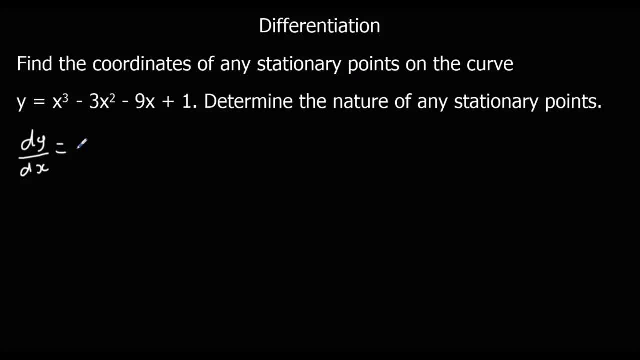 we're going to times by the power. take one off the power, So 3x squared minus 6x minus 9.. So there's our gradient function. We need to know where it's equal to zero. So we've got 3x squared minus 6x minus 9 equals zero. So we're going to solve it if we divide by: 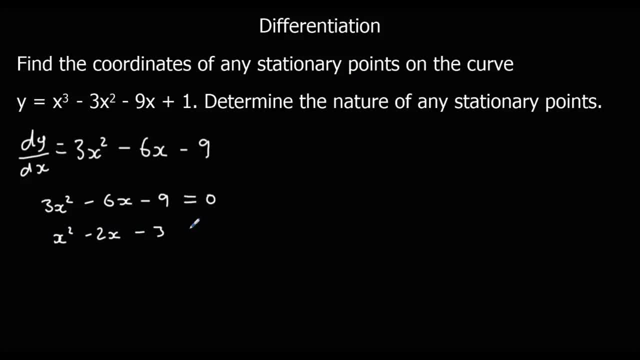 three first and then factorize it. So x is three and x is minus one. So they are the x coordinates of the stationary points. If we substitute these back into the original, we can find the y coordinates to go with them. So when x is three, 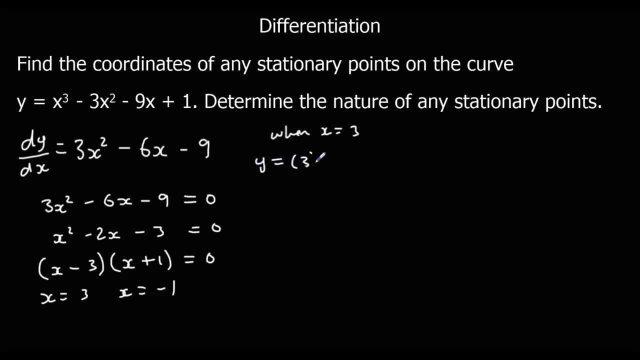 y is three cubed minus three, lots of three squared minus nine, threes plus one. So we're going to have 27 minus 27 minus 27 minus 27 plus one, which is minus 26.. So we've got a turning point at three minus 26.. And the other one when x is minus one. 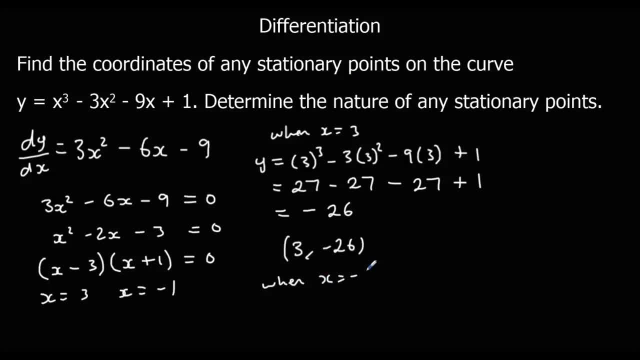 So when x equals minus one, we've got minus one cubed minus three. lots of three squared minus nine, threes plus one. So we've got minus one squared minus nine, minus ones plus one. So we've got minus one minus three plus nine plus one, which is six. 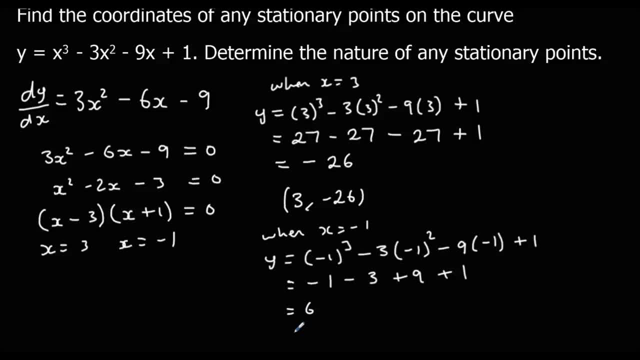 So we've got minus one six. So we've got the coordinates of our stationary points, but we still need to determine the nature of them. So what we need to do to determine the nature of stationary points is to do the gradient of the gradient. 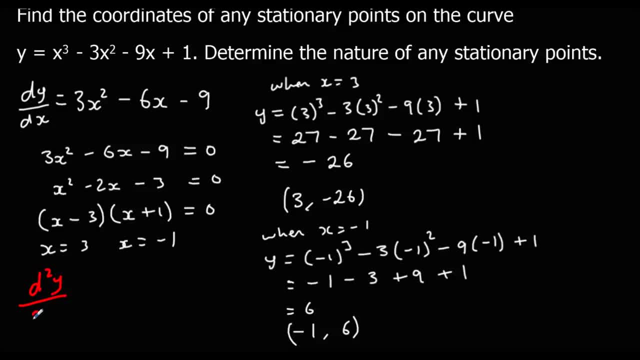 So we've got, this is the gradient. we're going to find the gradient of the gradient. So we're going to: times by the power- take one off the power. and times by the power: take one off the power, So that leaves us with six x minus six. 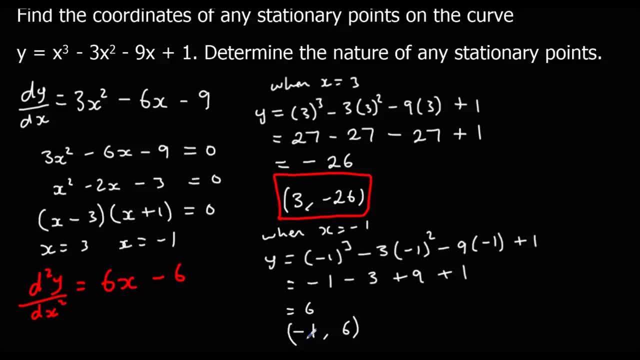 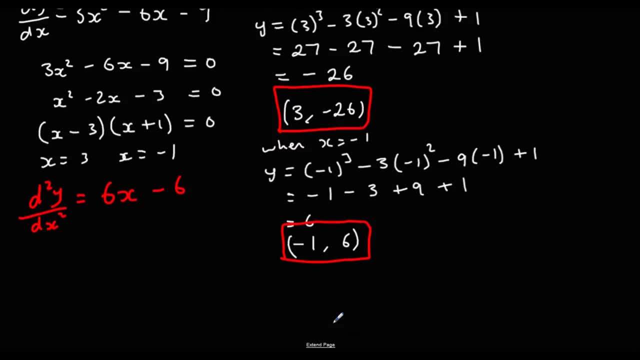 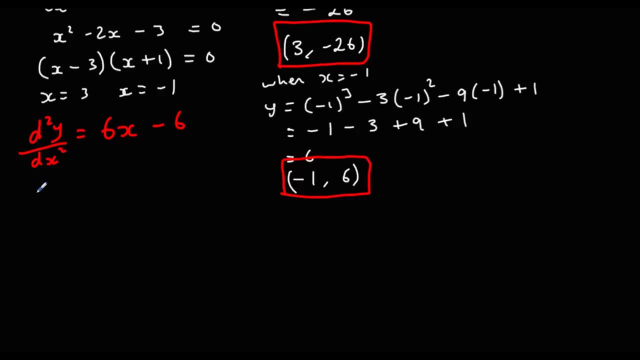 So we've got these two stationary points And we need to determine the nature of them. So all we're gonna do here for when x is three. So when x is three, the gradient of the gradient is six times three minus six. 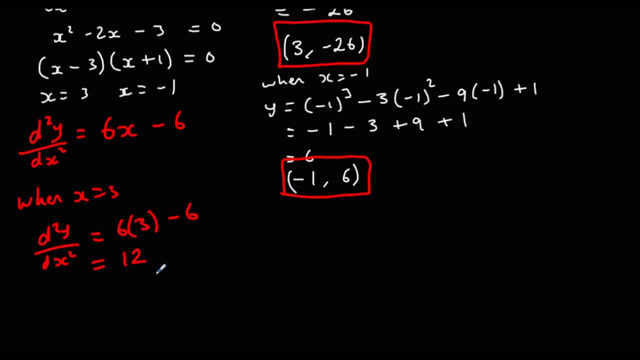 which is 12, so that's positive. so therefore it's a minimum. so this is a minimum, and exactly the same for this one. so when X is minus 1, the gradient of the gradient is 6 minus 1 minus 6, which is minus 12, so negative. therefore it's a maximum. so 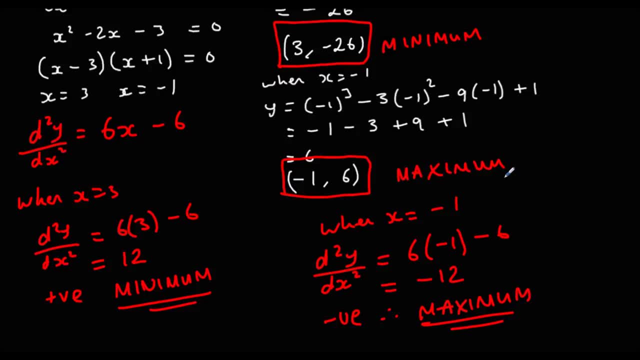 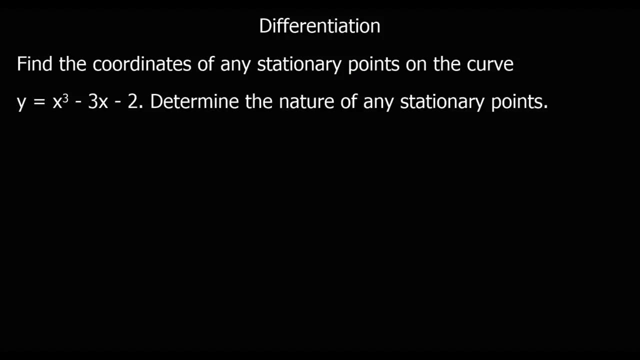 this one is a maximum. okay, here's another question. pause the video, try and see if you can do this one, and then I'll go through the answers after. okay, so again we need to find the coordinates of the stationary points. so that means find out where dy, dx, where the gradient function is 0. so we're. 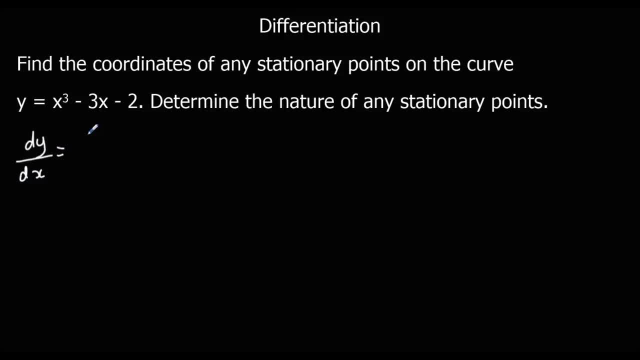 going to dy dx, and that's 3x squared minus 3 this time. where is it equal to 0? well, 3x x squared minus 3 is 0, so x squared minus 1, if I divide 3 by 3 equals 0, so if I factorise: 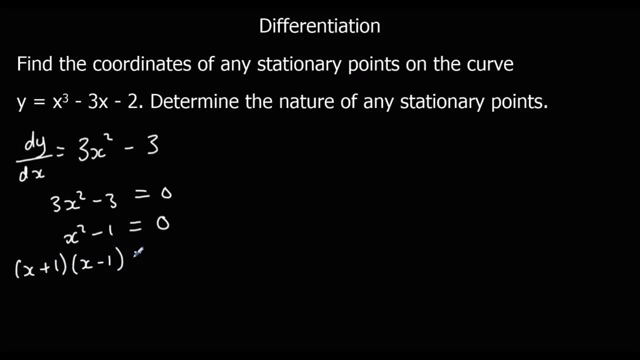 it. I've got x plus 1, x minus 1 equals 0 using the difference of two squares there. so x is minus 1 and x is 1.. It says coordinates. I'm going to find the y coordinates as well. 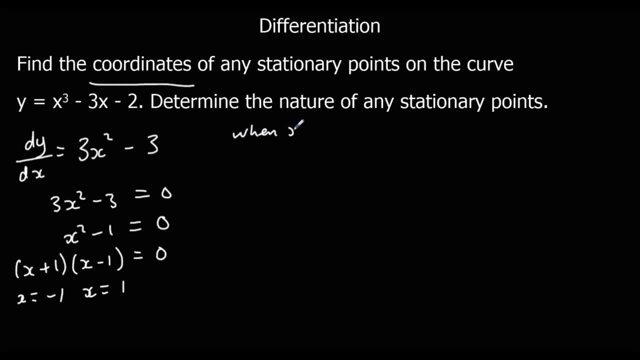 so when x is minus 1, y is minus 1, cubed minus 3 minus 1's minus 2,, which is minus 1 plus 3 minus 2, which is 0, so it's minus 1, 0..